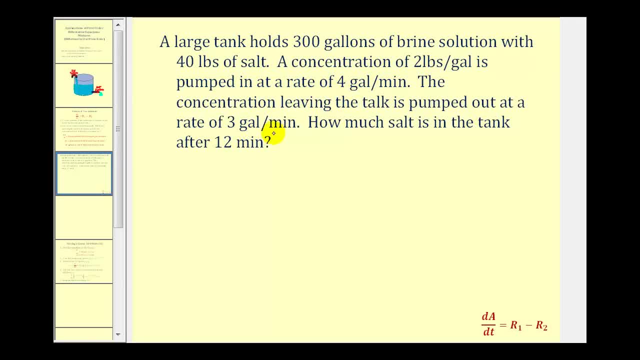 The concentration leaving the tank is pumped out at a rate of three gallons per minute. How much salt is in the tank after twelve minutes? So we're going to start with our differential equation. DADT equals R sub one minus R sub two, And we'll start by finding R sub one and R sub two. 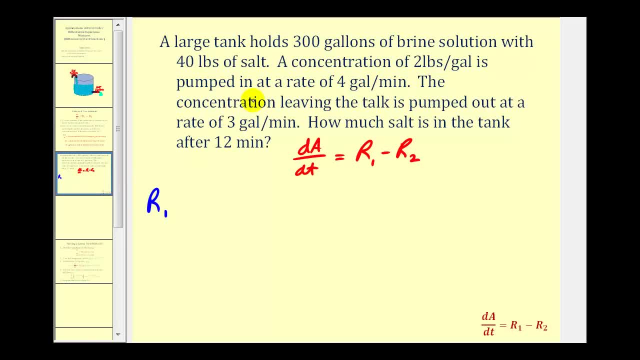 Where again, R sub one is the rate at which A of T is entering the tank and R sub two is the rate at which A of T is leaving the tank. Well, R sub one is pretty straightforward: We have two pounds per gallon pumped at a rate of four gallons per minute into the tank. So R sub one is: 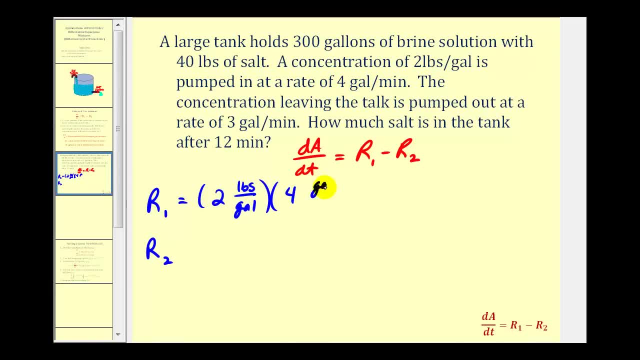 going to be the product of these two And I'm writing the units in fraction form so that we can see that the units of gallons simplifies out. So R sub one is going to be eight pounds per minute. Now. R sub two is going to be a little bit trickier because for the concentration, the amount of salt is. 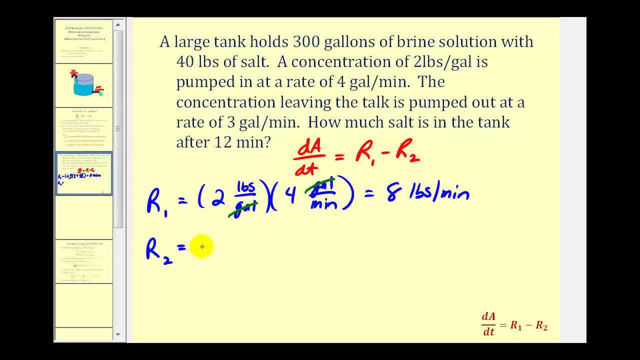 changing and so is the number of gallons in the tank. So for the concentration we're going to take the amount of salt and divide by the number of gallons in the tank. So A or A of T is the amount of salt in the tank. 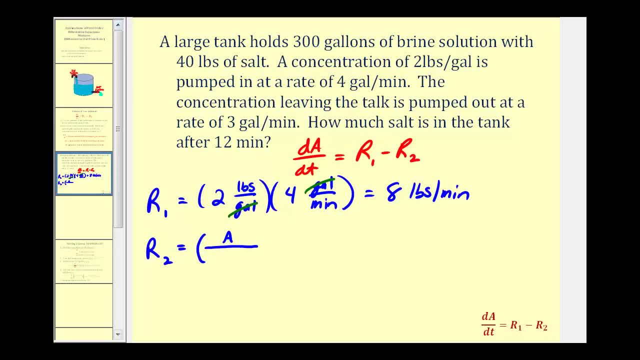 Now the number of gallons is not just three hundred, because notice how the solution is being pumped in at four gallons per minute and pumped out at three gallons per minute. So after every minute we have one more gallon in the tank, So the total gallons is going to be three hundred. 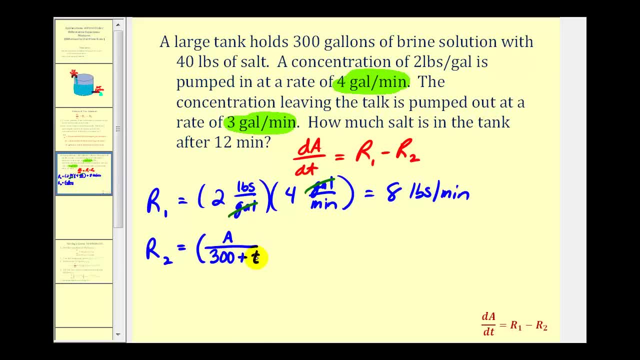 plus one T, where T is the number of minutes. Again, because we have one extra gallon every minute, we have one T here. This is going to be pounds per gallon times the rate of three gallons per minute. Again, gallons simplifies out. 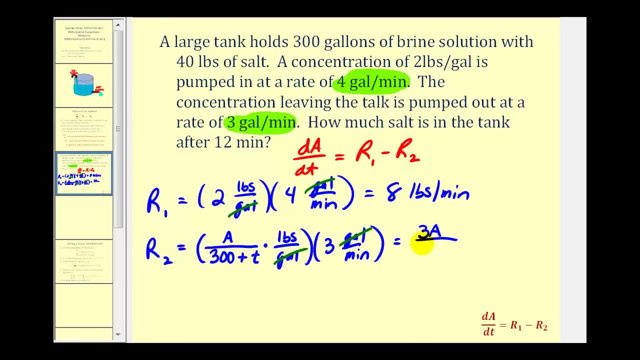 So R sub two is going to be three. A divided by three hundred plus T, and this would be pounds per minute. So the differential equation to model this situation that we need to solve is d A. d. T equals R sub one, which is eight. 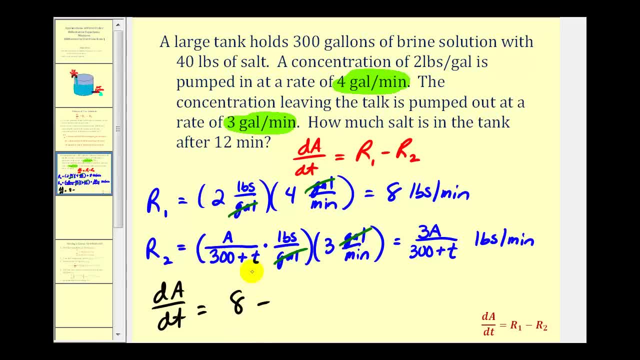 minus R sub two, which I'm going to go ahead and write as three divided by the quantity three hundred plus T plus T minus R sub two times A. The reason I'm writing it this way is it's easier to recognize that this is a linear. 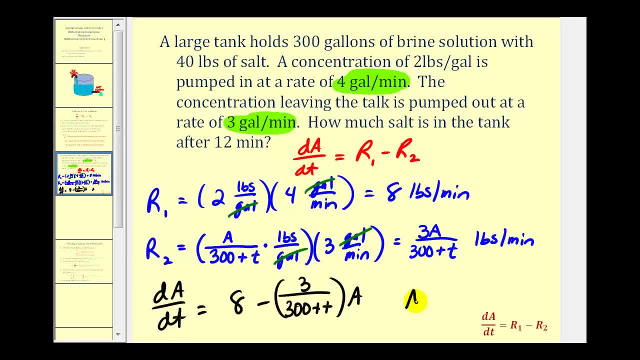 first order differential equation, And also we know that A of zero is equal to forty, because at time T equals zero, there's forty pounds of salt in the tank. Now we'll go ahead and solve this using an integrating factor. So the first step will be to write this in standard form: 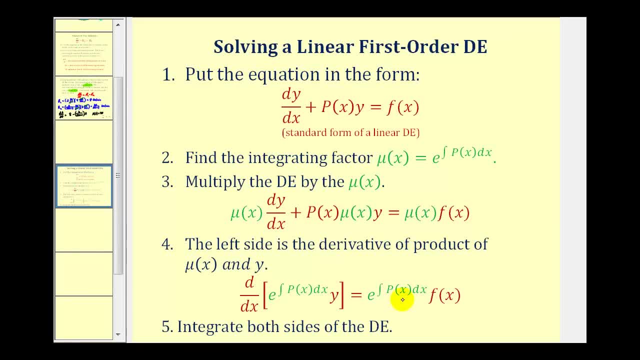 And for a quick review, you may want to pause the video on this slide to review how to solve a linear using an integrating factor given here, where P of X is the coefficient of our function Y or, in our case, the function A. 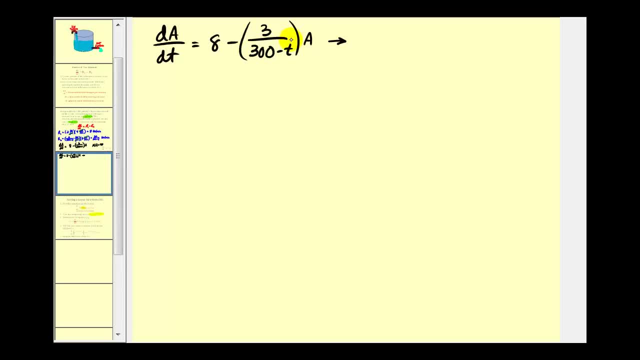 So to write this in standard form, we're going to go ahead and add this quantity here to both sides of the equation. So we'd have d A, d, T plus three. divided by three hundred plus T times A equals eight. So here's our function: P of T. 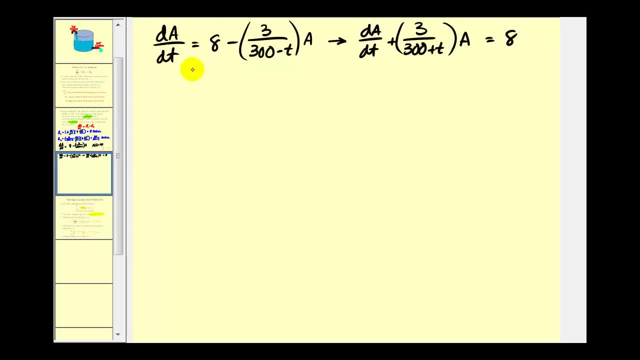 that we'll use to find the integrating factor. So the integrating factor- we'll call it mu of T, is going to be equal to E raised to the power of the integral of this function here, three divided by three hundred plus T d T. 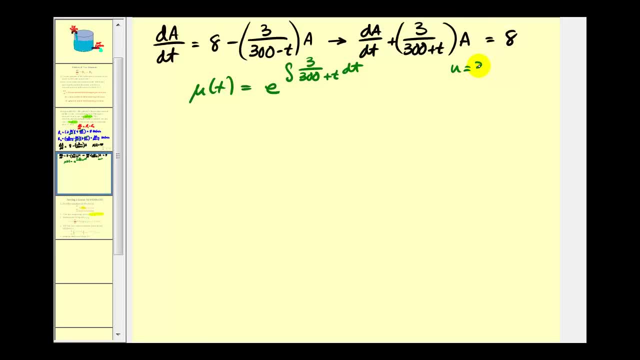 So to integrate this, we go ahead and let U equal the denominator of three hundred plus T And notice that d? U is equal to d T, So this just ends up being E. raised to the power of this would be three times natural log. 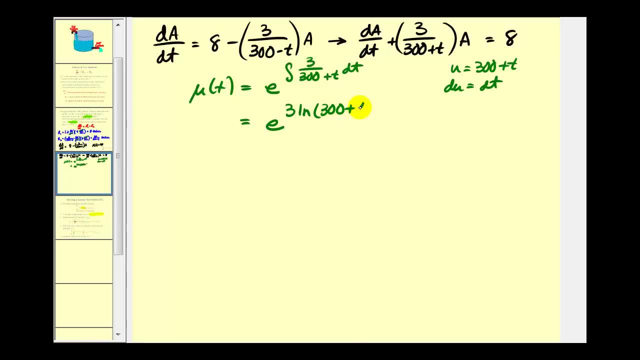 of the quantity three hundred plus T. We know T is always positive, so we don't need absolute values here, And from here we can use our property of logarithms to move this three here to the position of our exponent. So now we have: 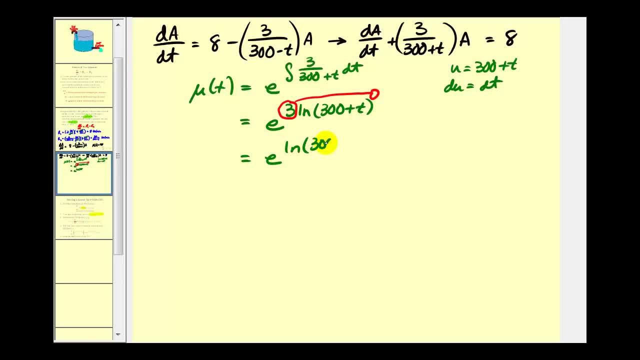 E raised to the power of natural log times, the quantity three hundred plus T to the third. This simplifies very nicely because we have base E here and this is natural log or log base E. So our integrating factor is just the quantity three hundred plus T. 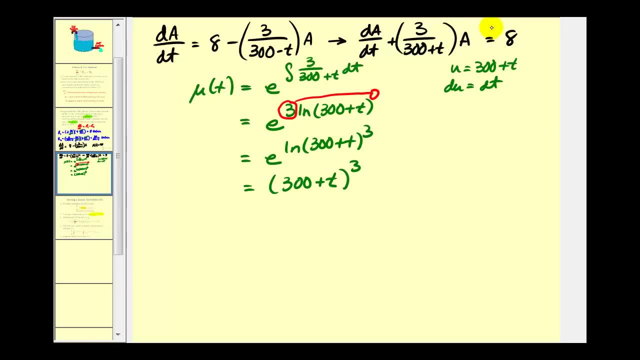 raised to the third. Now we'll take this form of our differential equation and multiply everything by our integrating factor. Now remember, when we do this, the left side of this differential equation, or this side here, is equal to the derivative of the product. 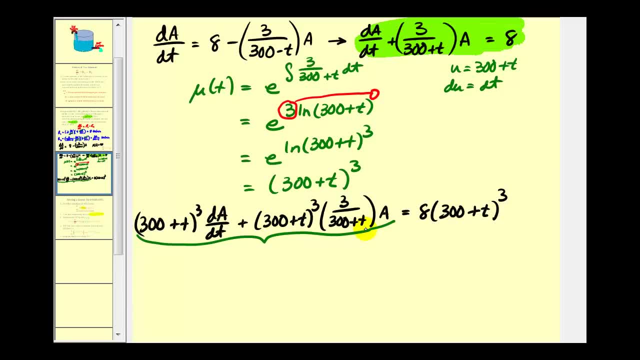 of the integrating factor and our function A. So we can say the left side is equal to the derivative of our integrating factor, which is three hundred plus T to the third times our function A or A of T. And we can verify this using the product rule. 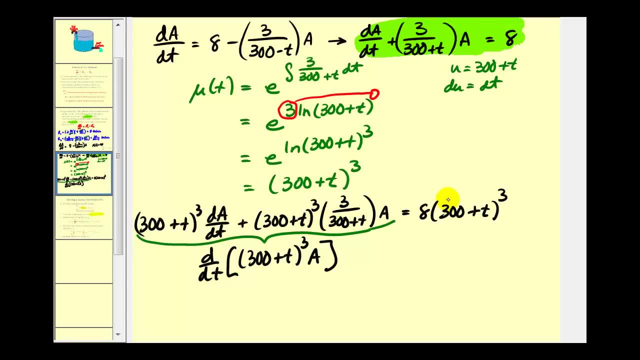 But if the derivative is equal to the left side of this equation, it must also equal the right side. so this is equal to eight times the quantity three hundred plus T raised to the third, And from here we can now integrate both sides of this equation with respect to T. 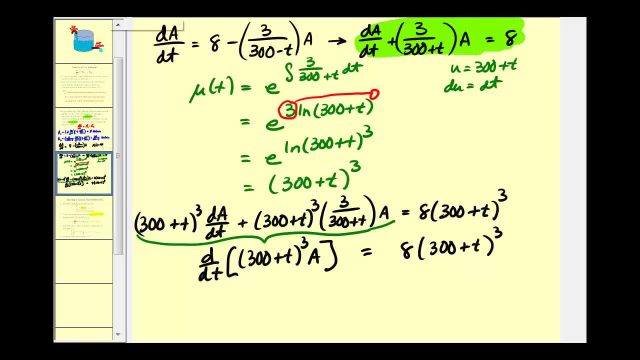 and then solve for our function A. So now we're going to integrate the left side and integrate the right side. On the left side the integral and derivative undo each other. so we're left with the quantity three hundred plus T to the third times A. 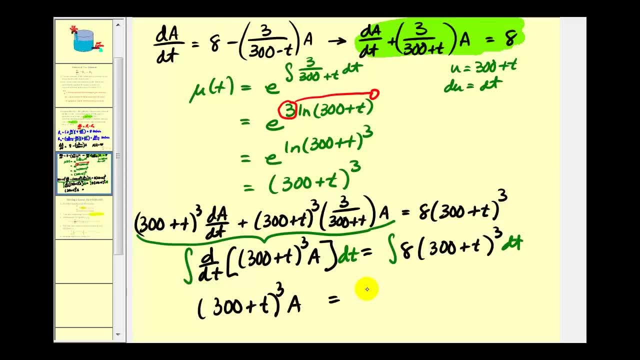 And then on the right side, if we integrate this, we would have eight times three hundred plus T to the fourth, divided by four plus C. Notice how the eight and the four simplify nicely. Let's continue this on the next slide. 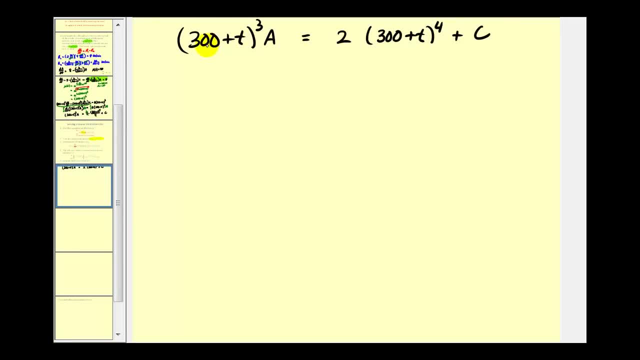 And now to solve for A, we'll divide by this quantity here. So on the left side this simplifies to A or A of T. On the right side, notice how all of this simplifies to just one factor of three hundred plus T. 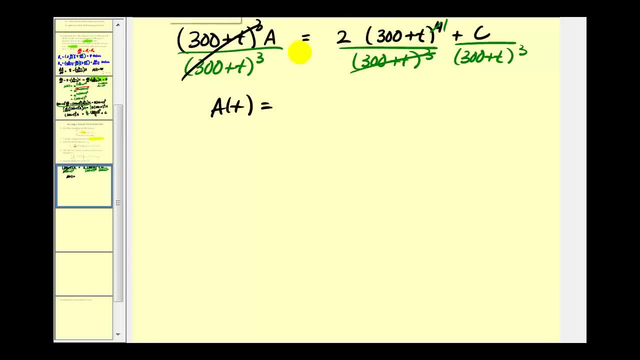 We'll go ahead and distribute the two. that would give us six hundred plus two T plus here. we'll go ahead and move this up into the numerator, which would change the sign of the exponent. So we'd have C times three hundred plus T. 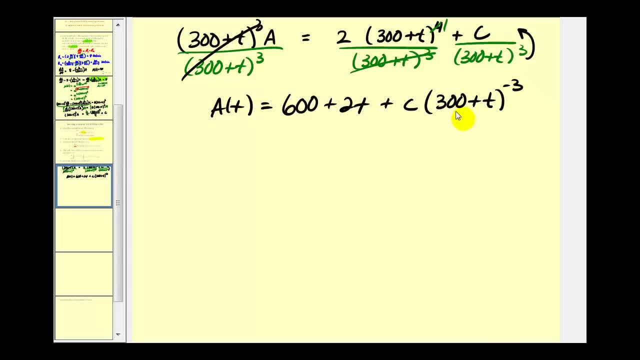 to the negative. third, This would be the general solution to our differential equation, but remember we also know that A of zero is equal to forty, So this will allow us to find our constant here and find our particular solution for this differential equation. 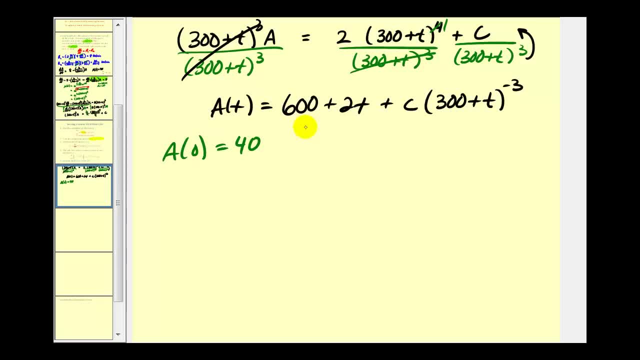 So if A of zero is equal to forty, we'll substitute zero for T and then set this equal to forty, So we would have six hundred two. T would be zero, so we'd have six hundred plus C times. this would just be three hundred. 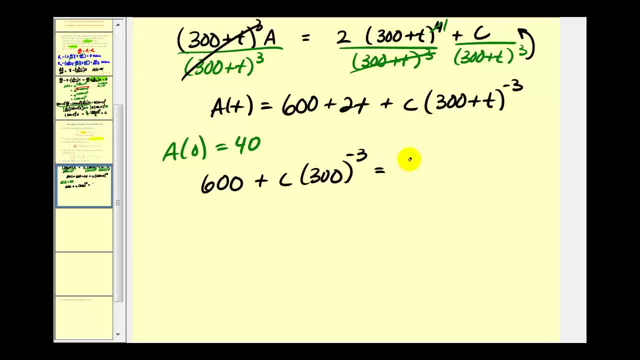 to the negative third power, and this equals forty. So next we would subtract six hundred on both sides. that would give us negative five hundred sixty. Now here we could divide by three hundred to the negative third, or just multiply by three hundred to the positive third. 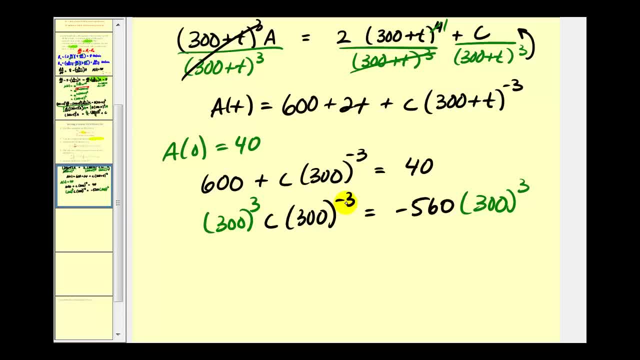 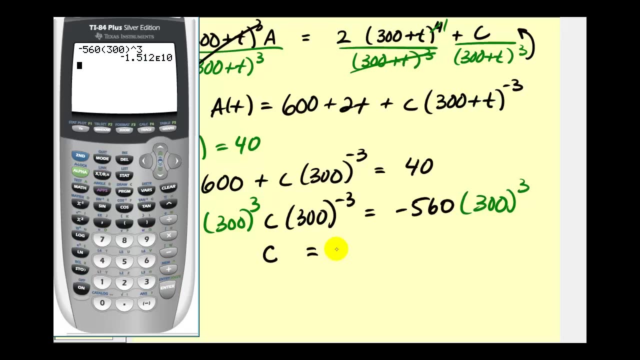 Remember, here we'd add the exponents. that would give us three hundred to the zero, which is equal to one. So we have C equals this product here, which we'll go to the calculator for We have negative one point five, one, two times ten to the tenth. 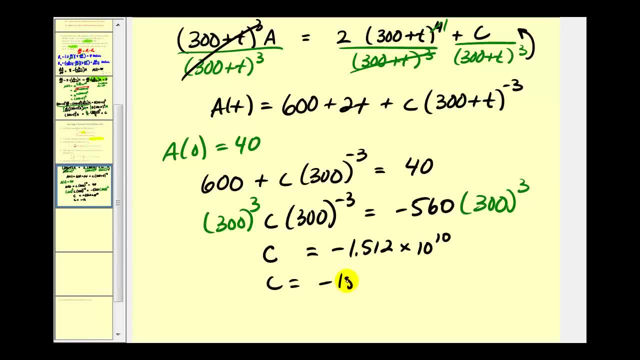 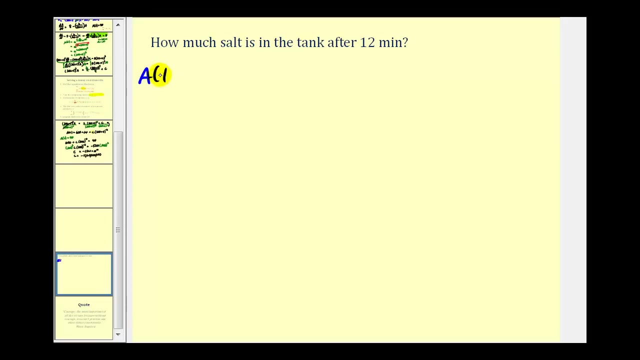 Using decimal notation, we'd have negative one, five, one, two. we need seven more zeros. So we have negative fifteen billion, one hundred twenty million for our constant C, Which we'll now substitute back into our function A of T for C. So we have A of T. 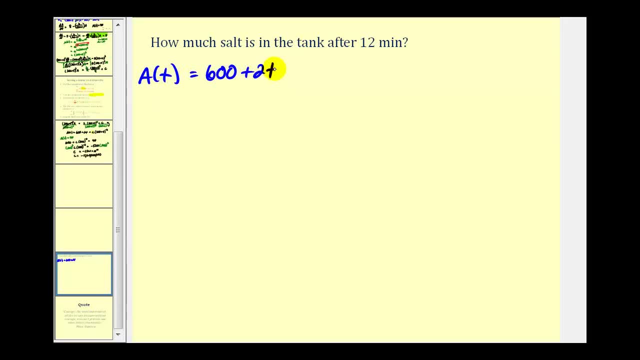 equals six hundred plus two T minus fifteen billion. one hundred twenty million times three hundred plus T to the negative third power. So now to answer the question: how much salt is in the tank after twelve minutes? we need to find the value of A of twelve. 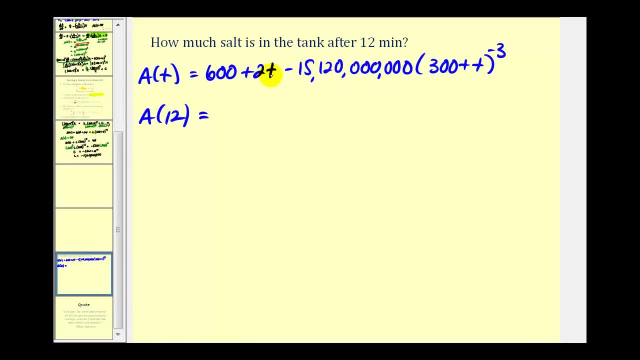 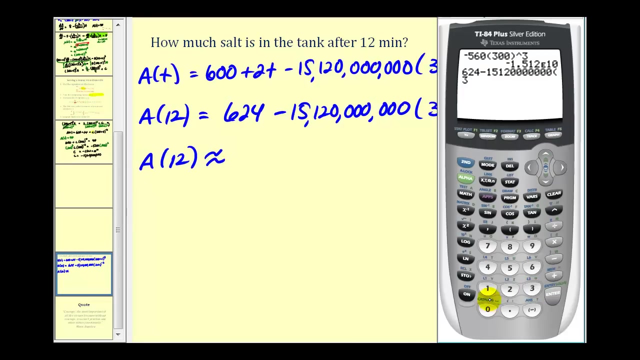 So we'll substitute twelve for T. this would be six hundred plus twenty four. six hundred twenty four minus fifteen billion. one hundred twenty million times this would be three hundred twelve to the power of negative three, And we'll go back to the calculator.